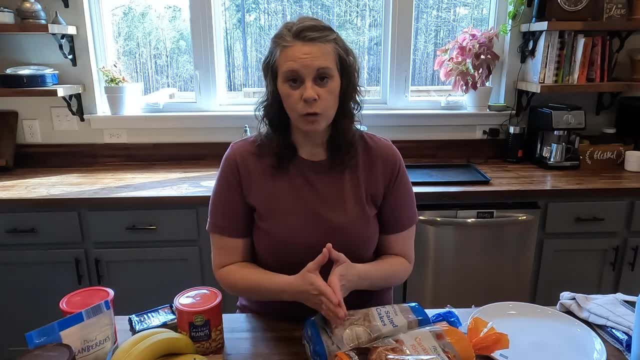 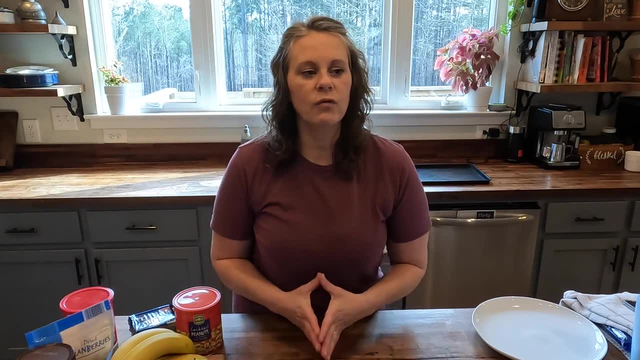 inexpensive and helpful items to have in your pantry. But sometimes even those pre-packaged items don't really hit the spot or it's not exactly what you're looking for. So I want to give us a couple of ideas that we can go to on a regular basis to have. 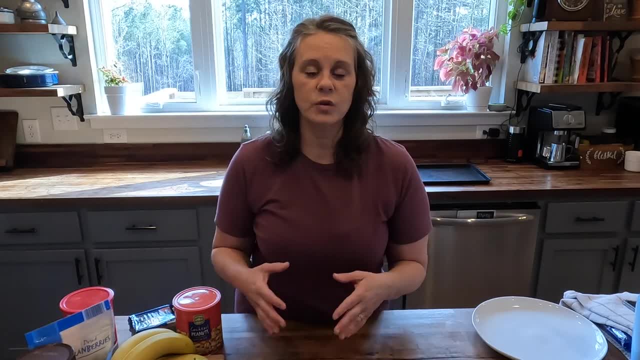 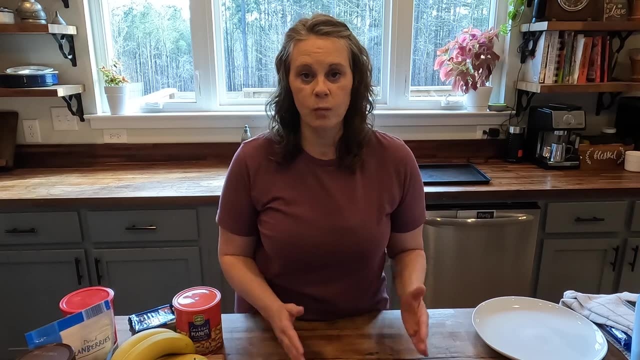 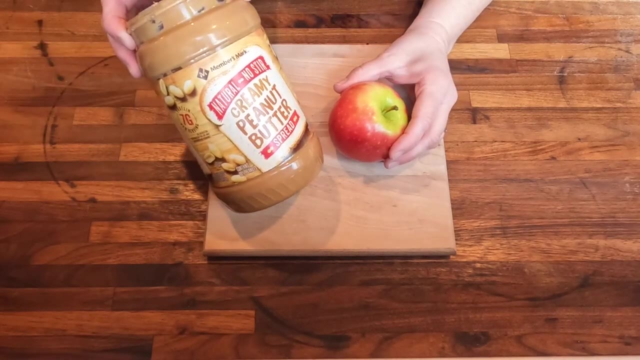 some inexpensive, easy go-to snack options that our family is going to enjoy and also is not going to break the budget when we go to the store and purchase them week by week. First of all, let's talk about the amazing combination of apples and peanut butter. I think pretty much. 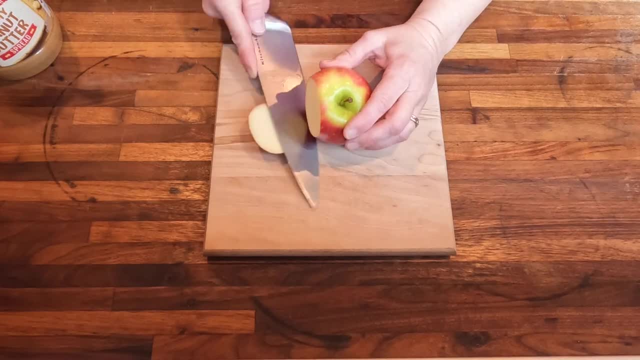 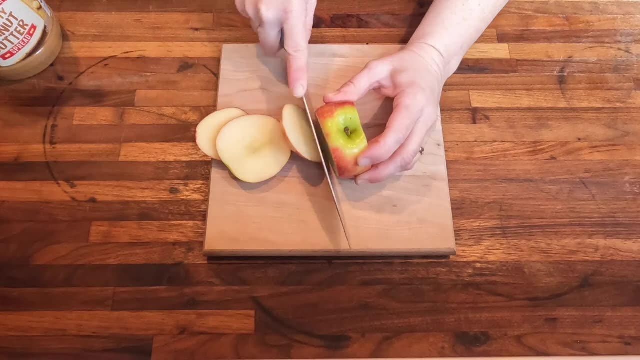 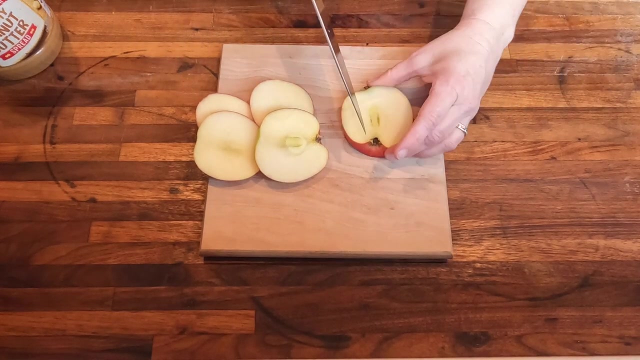 everybody is a fan of this if they like peanut butter, And this makes for a very simple and easy snack that pretty much everybody is going to enjoy. I know there are some peanut allergies out there that we have to be concerned about, but I think that we have done a much better job. 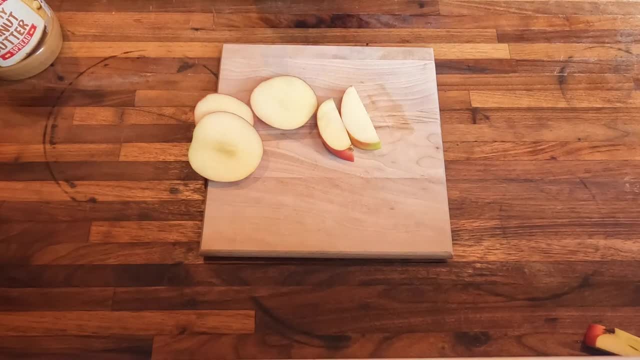 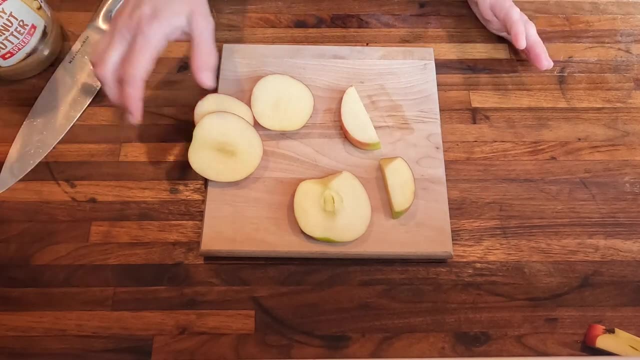 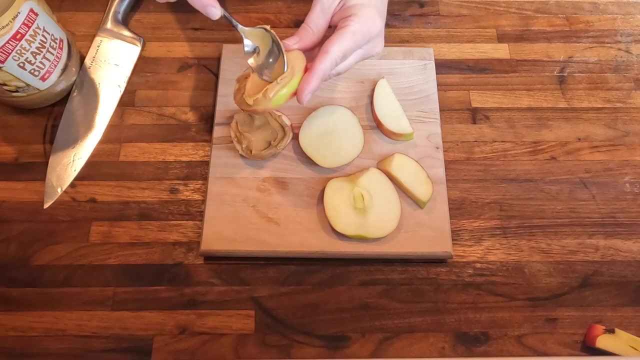 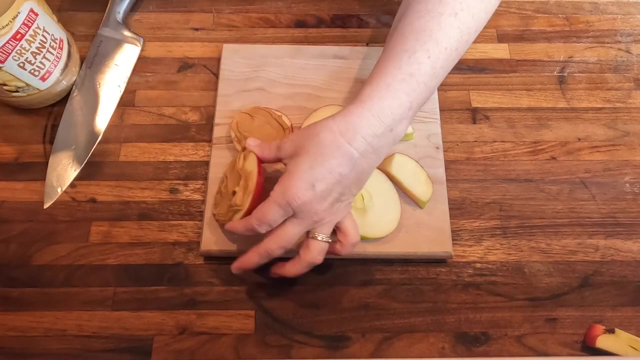 of getting a handle on those allergies by introducing nuts and nut butters to kids a lot earlier than we previously had. They have found that if you introduce nuts or nut butters before their first birthday, the chances of them adopting a peanut allergy or a nut allergy in general is. 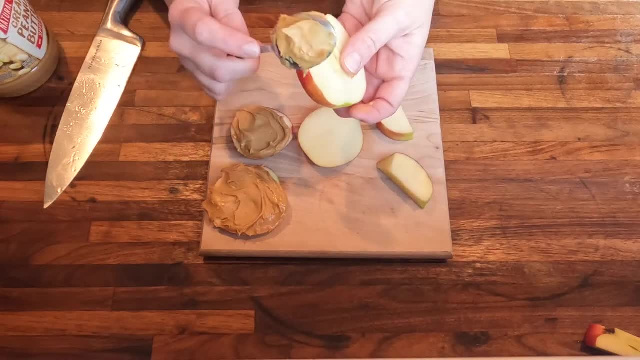 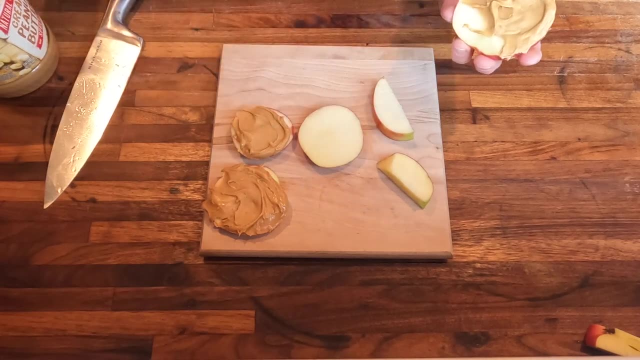 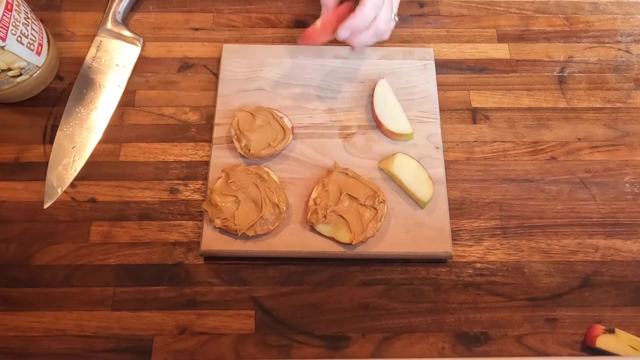 very much reduced, So even your little kids can enjoy this snack. but if Lane was eating this- since he's still pretty young and I'm really afraid of him choking on things- I would peel the apple before I gave it to him. That way it would be a lot safer for him. So I'm just going to cover. 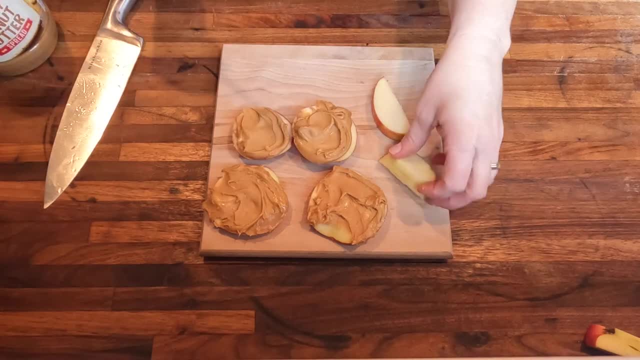 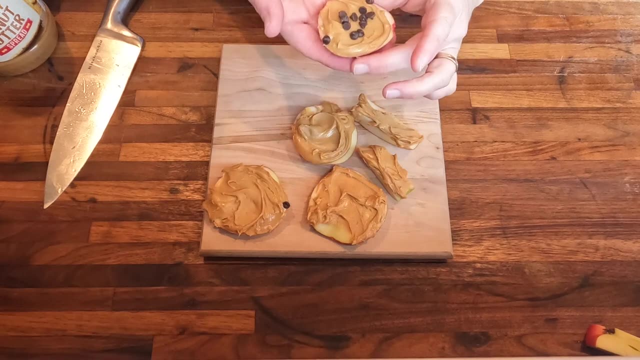 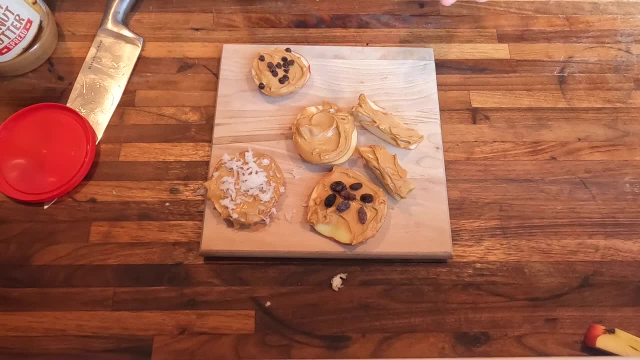 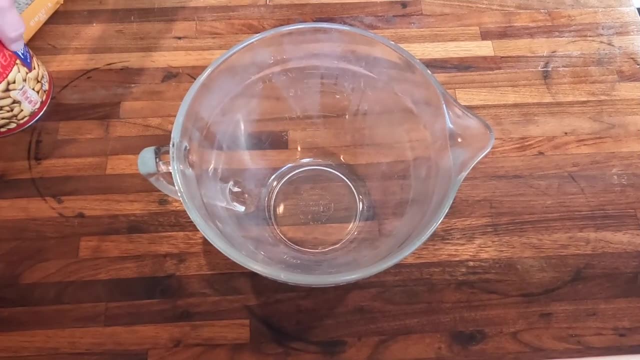 There are so many options: granola, bananas, all kinds of options to spruce up your peanut butter and apple snack. Another really good option for a quick and filling snack is to have a little bit of peanut butter on top of your peanut butter and peanut butter. 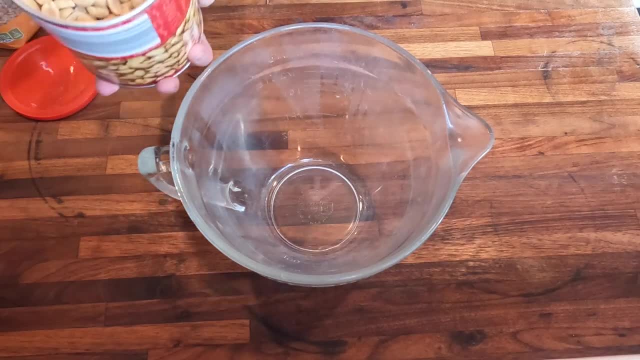 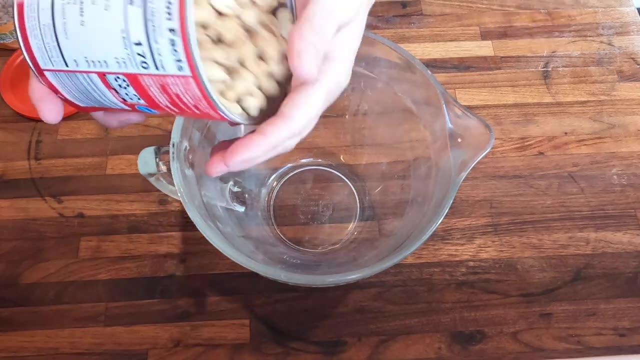 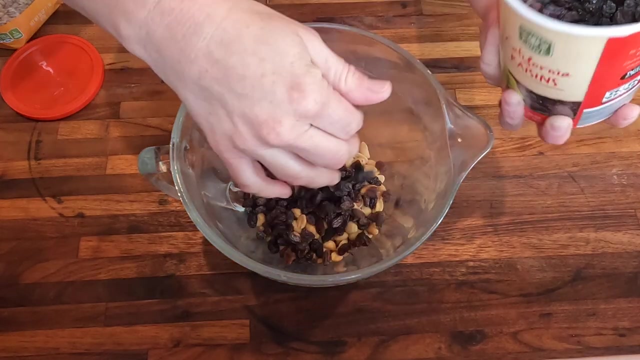 To make your own trail mix. you can do so many things with trail mix, So I'm just going to throw a couple of ingredients together just to give you some ideas. There's no need to measure, So I have just some inexpensive cocktail peanuts. I'll add some raisins, some cranberries. 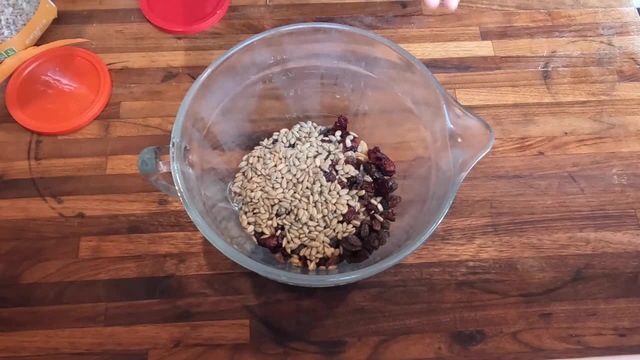 some sunflower seeds. And to add a little bit of sweet to the salty, I'll add some semi-sweet chocolate chips. I'm going to add a little bit of sugar. I'm going to add a little bit of salt. I'm going to add a little bit of sugar. I'm going to add a little bit of sugar. I'm going to add a little bit of sugar. 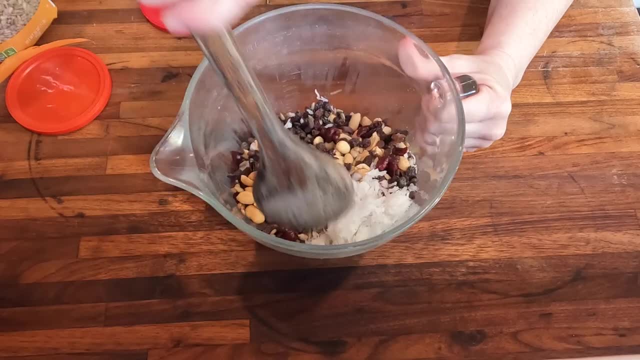 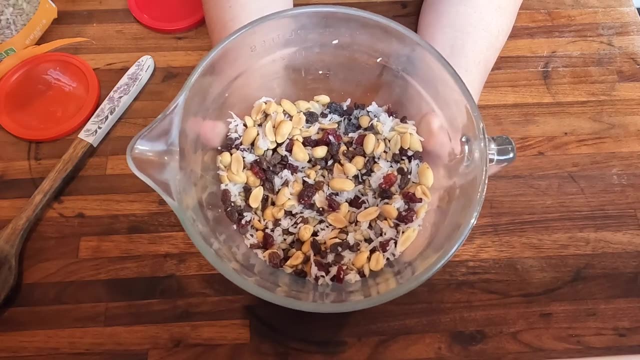 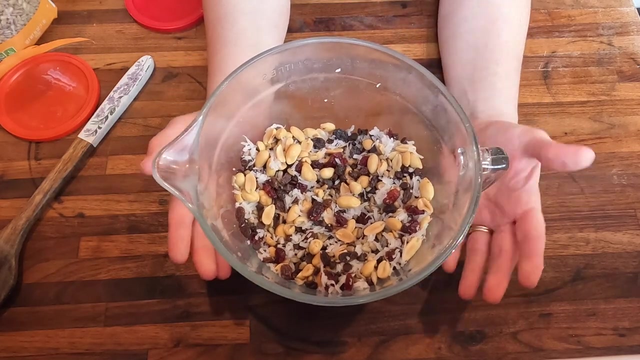 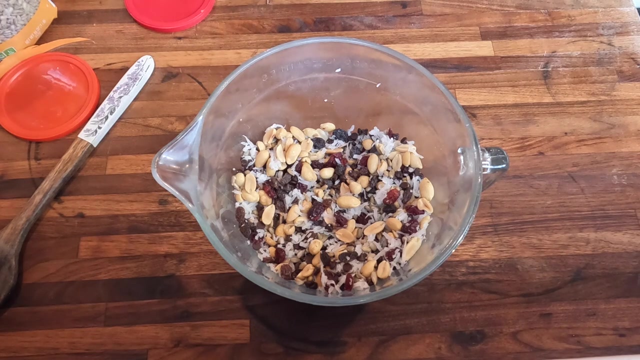 Maybe even some of that coconut. Give that a good stir. If you put this into individual baggies or into an airtight container, it will stay good all week, And so you will have made a delicious, nutritious, protein-filled snack with very little effort and also minimal cost. 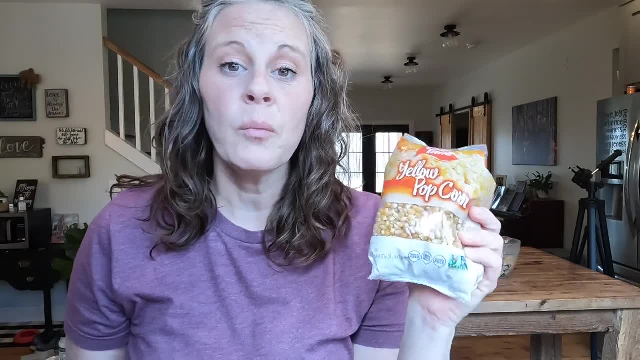 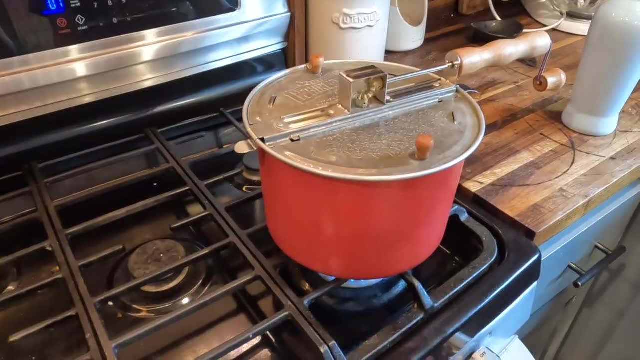 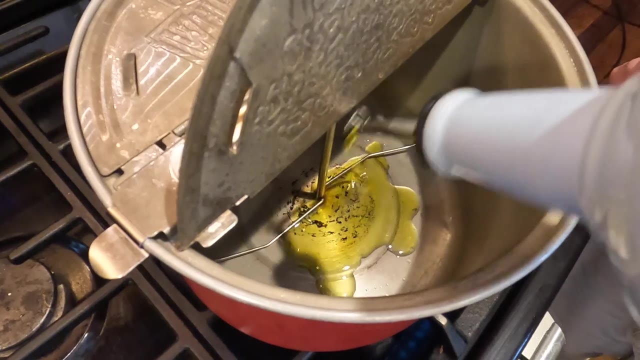 One of my family's very favorite snacks is popcorn. It could not get any simpler than pouring a little bit of popcorn and oil in one of these popcorn poppers. They sell all of the ingredients at the Dollar Tree. I will link this popper down below on Amazon. You can go and check it out. I have bought. 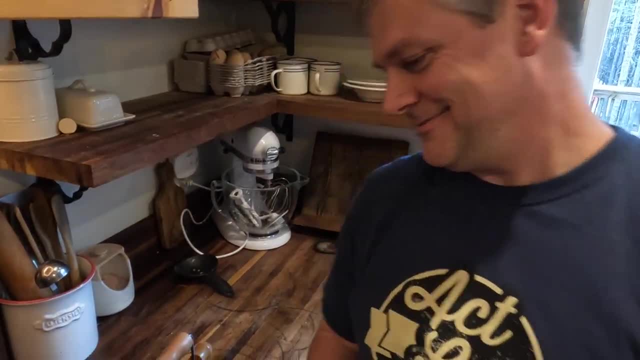 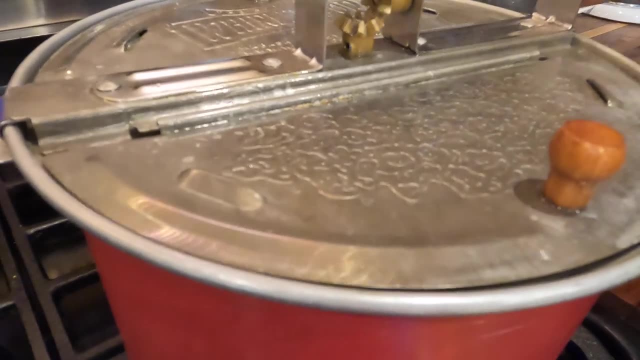 fancy popcorn poppers for Chris, because he literally loves popcorn. We eat it almost every day. But the fancy, expensive popcorn poppers are not as good as this Warley Pop. It's a pop that we have had for years and years. It stands up under a lot of abuse. 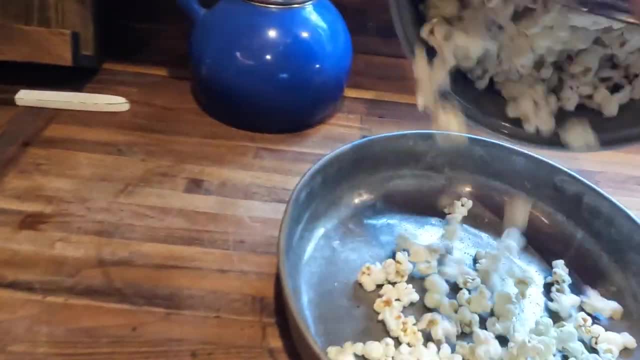 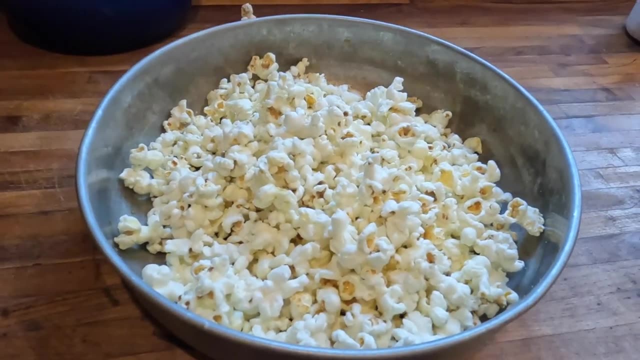 and we love the taste of the popcorn that we get from the Warley Pop popper. I know a lot of people enjoy the air-popped popcorn, but I just feel like there's no comparison in the flavor that you get if you cook popcorn in olive oil on the stove. 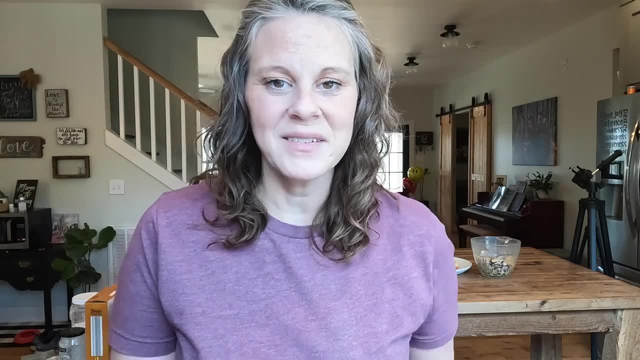 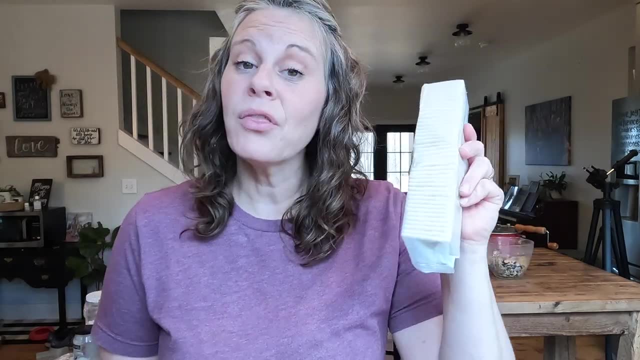 So that is a definite go-to for us. When you talk about inexpensive snacks, it doesn't get much cheaper than a box of popcorn. It doesn't get much cheaper than a box of popcorn. I have three ideas to spruce these crackers up, to give you some delicious snack options. 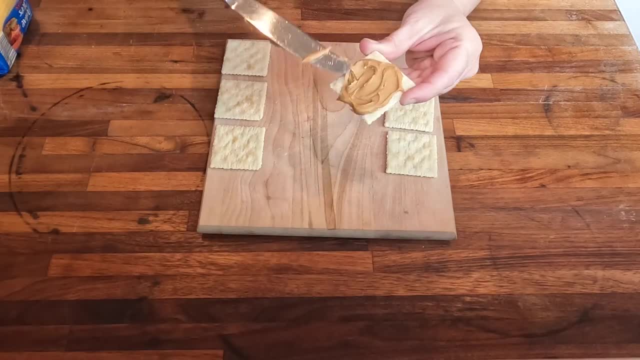 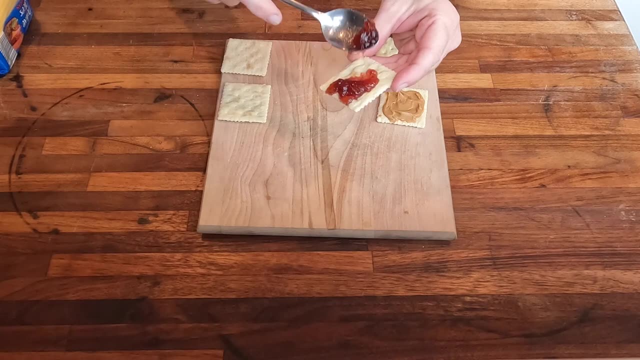 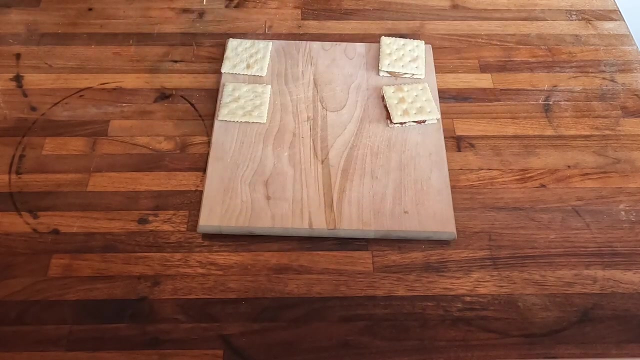 First of all, just a simple peanut butter cracker is portable, quick and easy. If you want to, you can add a little excitement to the plain peanut butter cracker by adding some jelly for a yummy PB&J cracker And also this deluxe cheese from Aldi. They also sell it at Walmart. 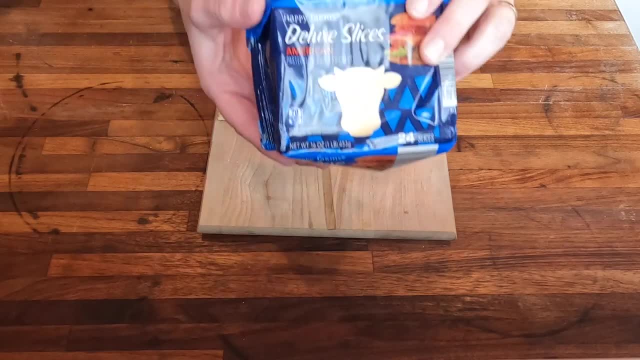 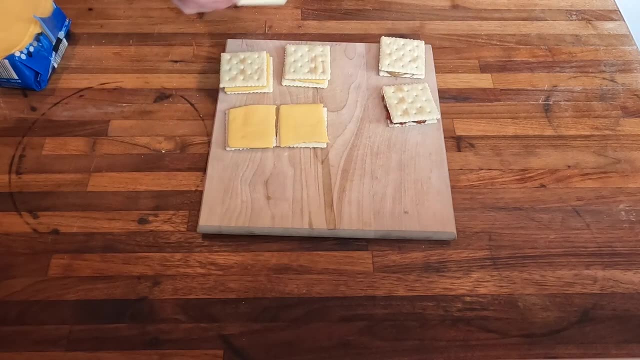 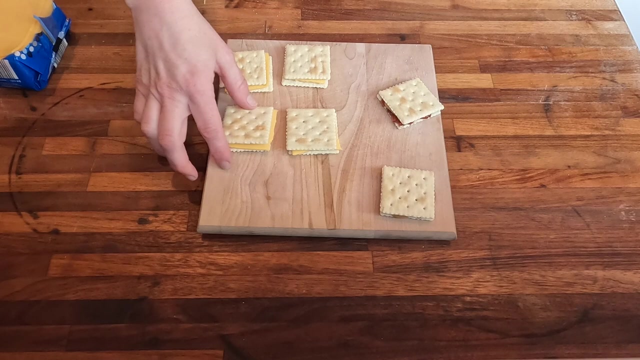 Kraft makes a more expensive version of it, but we really like this cheese And if you just fold it in half and fold it in half again, you have enough to make four cheese crackers. This whole box of crackers was a dollar, so you could feed your kids all week with these simple. 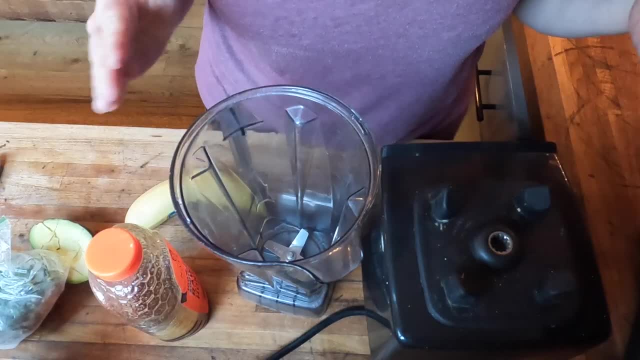 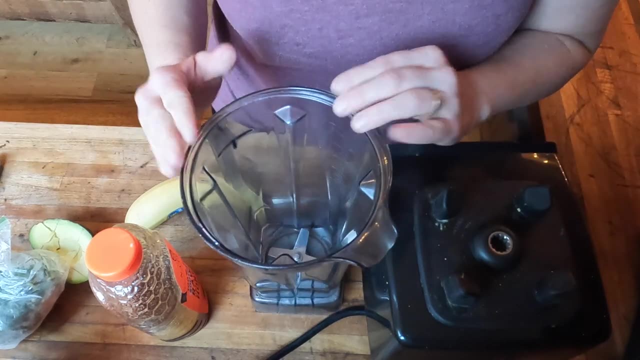 and affordable snacks. Another great option for a snack that is both healthy and filling is a smoothie. If you have a high-speed blender, you can use a blender to make a smoothie. This is simple and easy and quick to do. You can also just use an immersion blender. 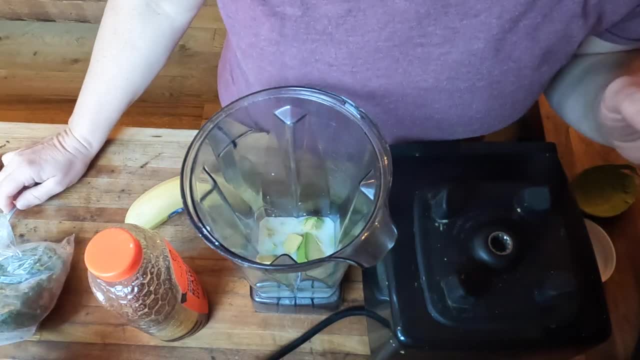 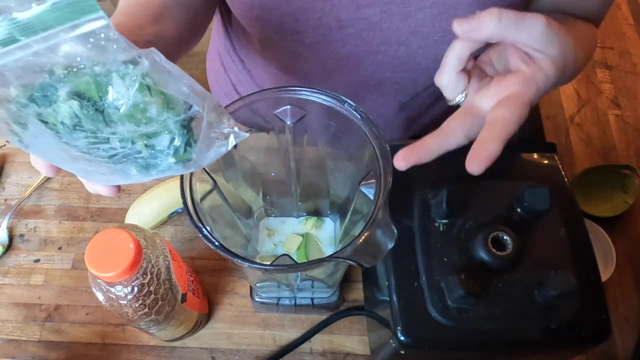 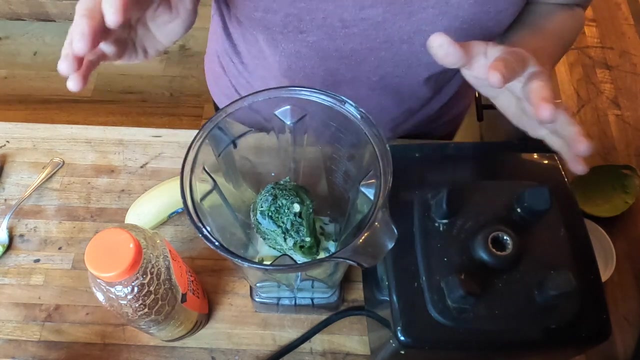 I'm just going to add a little bit of milk, half an avocado. I have taken a package of spinach and a package of kale. I separated them into individual servings and I froze them in little sandwich bags And that just makes it quick and easy to add some. 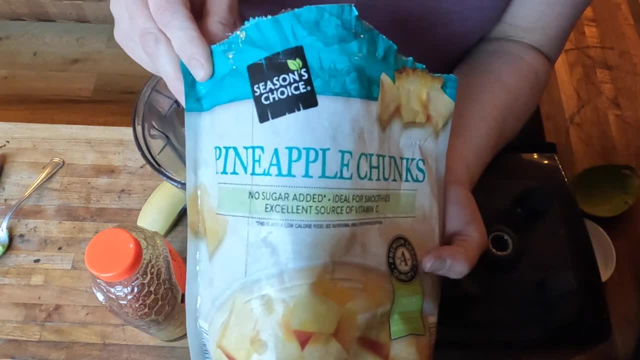 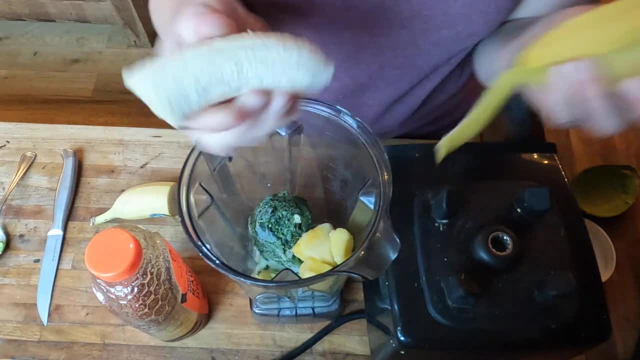 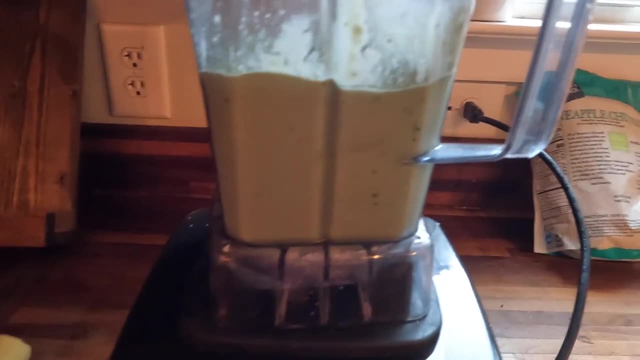 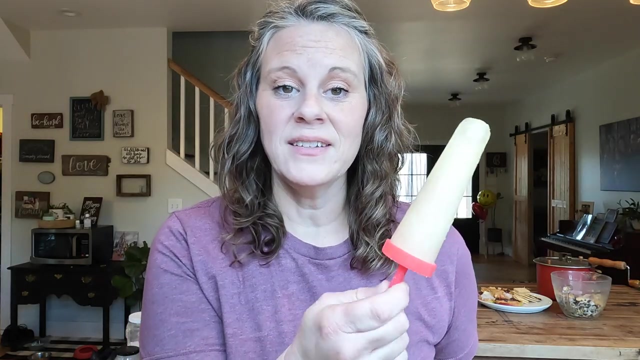 Just add a few of those: half a banana and about a tablespoon of honey. Even though it's not quite summer, it's always a good day when Lane gets one of these homemade apple juice popsicles. Even though it's not quite summer, it's always a good day when Lane gets one of these. 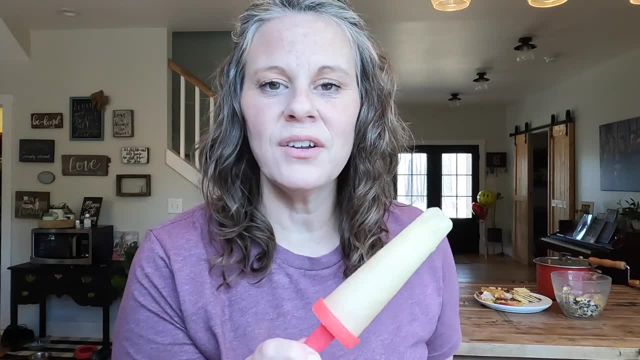 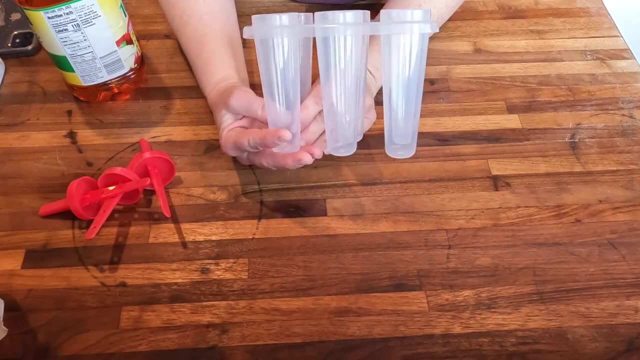 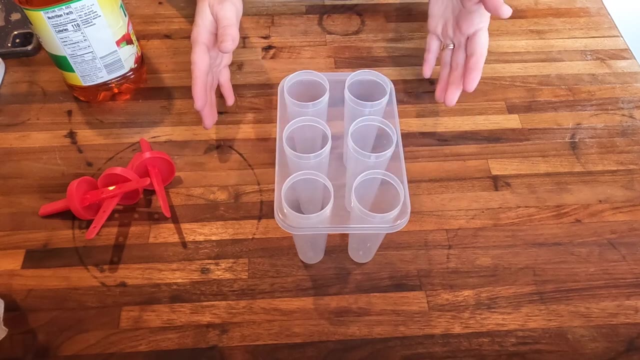 It doesn't matter how cold it is outside. He always thinks that they're in season and they are super easy and affordable to make. I couldn't find this exact popsicle mold on Amazon. This is a core brand I got at Ollie's. I don't know if y'all have an Ollie's near you, but if you do. 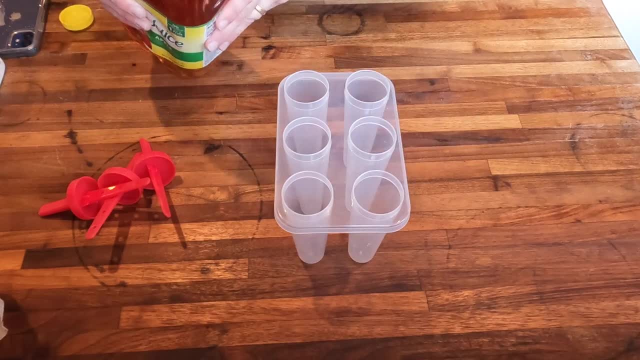 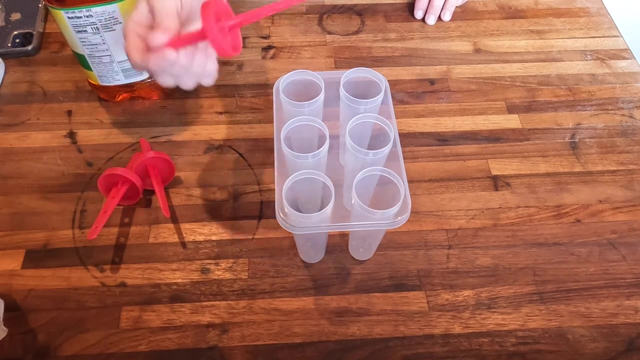 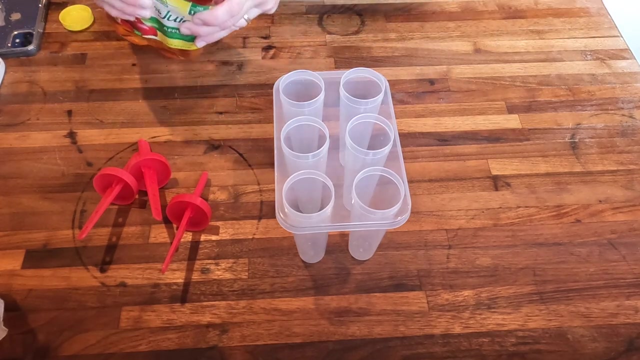 I would highly recommend that you go and check it out, But I will link one similar to this, because we had a different kind last year and this shape just really works a lot better for at least for Lane and the size that he is now Super easy, self-explanatory. 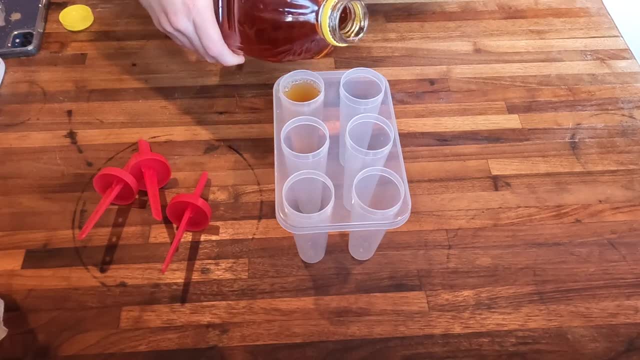 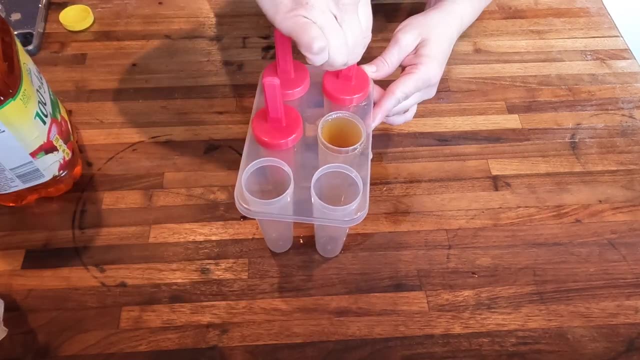 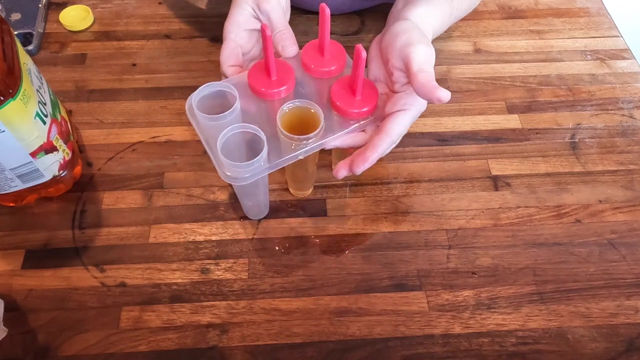 just to fill it up to the line with your choice of juice. You can also dilute it with water if you choose. Press the handles down in, put it in the freezer, freeze for four hours and you have some inexpensive popsicles. The reason that I decided to get these popsicle: 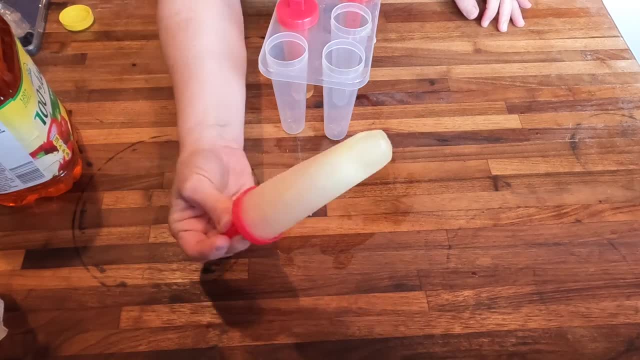 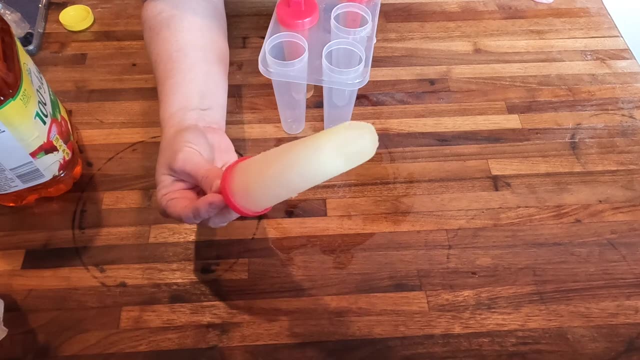 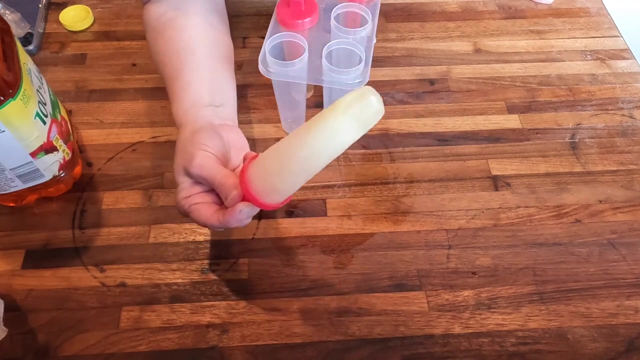 molds and make my own was. I read the ingredients on the box of popsicles that's available at the store And if you don't want to pay $6 for four popsicles, then you're going to get a lot of artificial dyes, artificial sweeteners, all kinds of things that I just didn't want Lane to be. 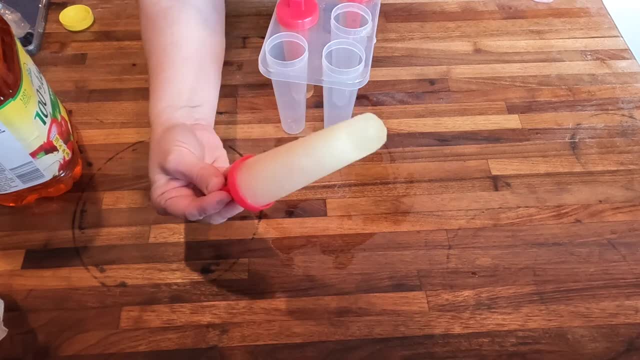 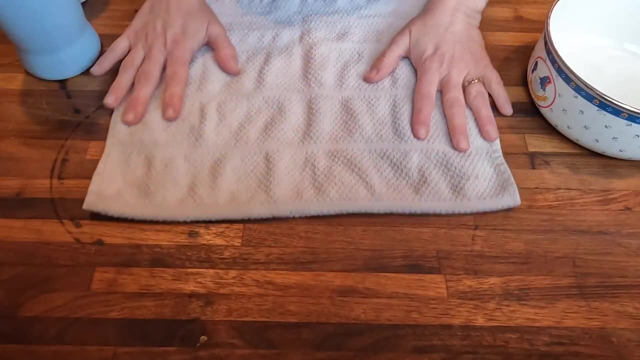 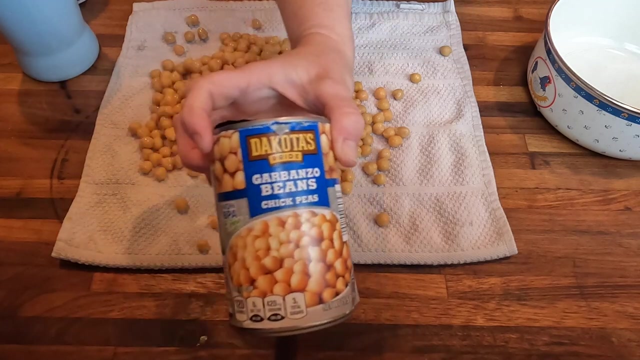 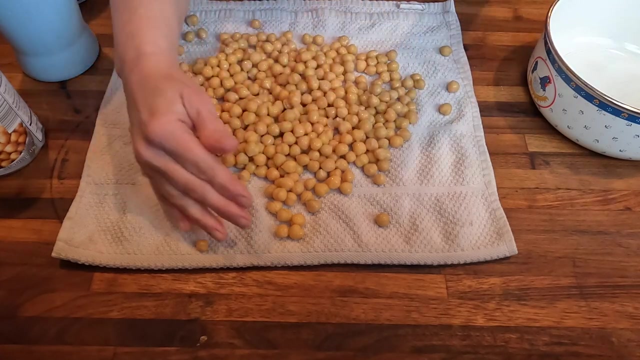 eating, Especially when he was eating three popsicles a day. So this has really been a big money saver for us. Next up, let's make some roasted chickpeas. Super simple recipe. I've got two cans of garbanzo beans chickpeas and I have drained them and rinsed them, And now I'm just 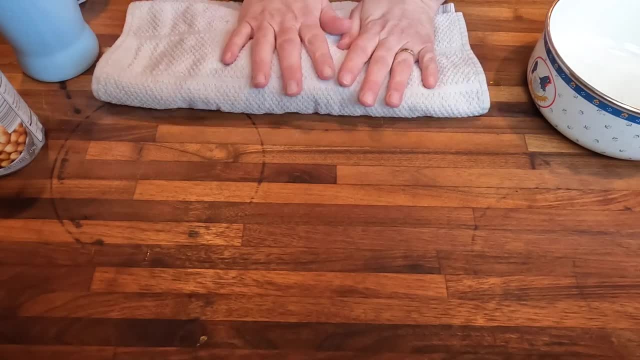 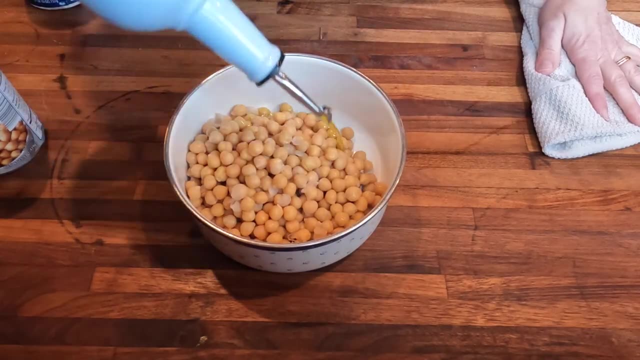 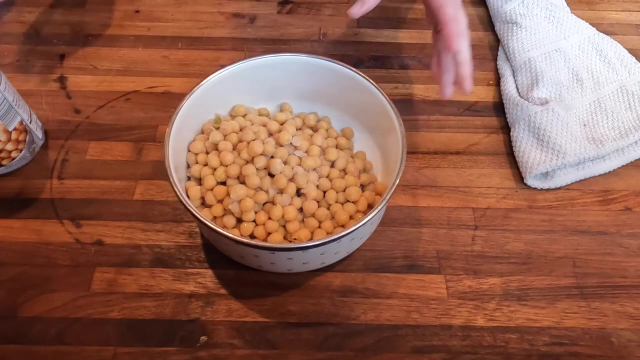 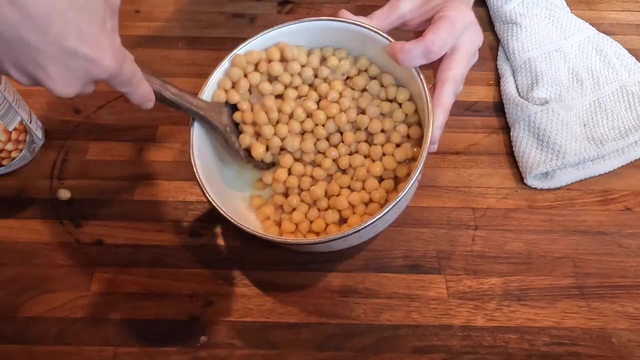 going to sort of pat them dry on this clean towel. I'm going to pour them into a bowl And add about two tablespoons of olive oil and sprinkle some salt. You can also use chili powder. You can use garlic powder, cumin, any kind of seasoning that you like. 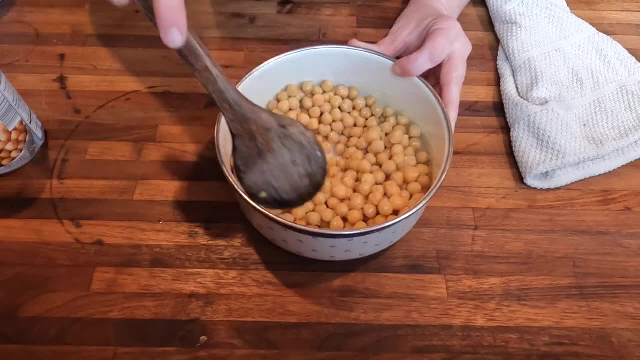 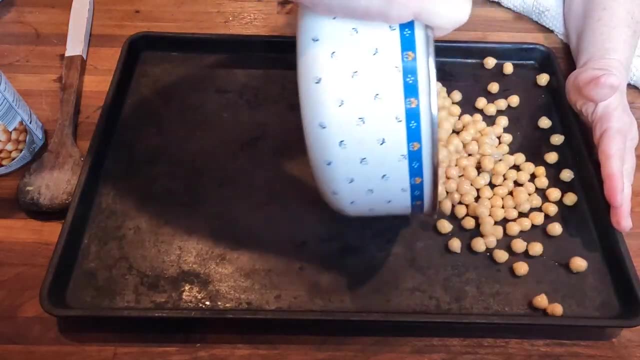 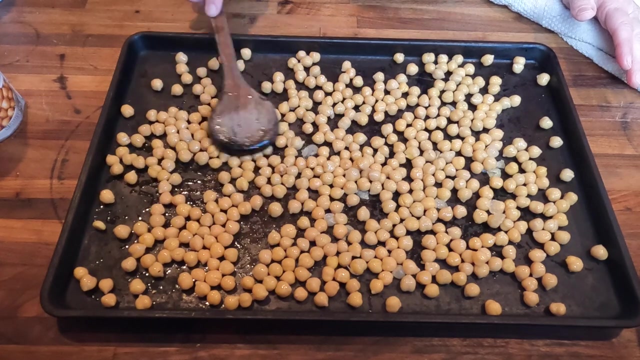 I'm just going to keep these simple so the kids will be more likely to enjoy them. Make sure they're all well-coated with that oil. I'm going to spread them out on this cookie sheet. I have the oven preheated to 400 degrees. They will cook for about 25 to 30 minutes at 400 degrees, with me stirring them and rotating them every five minutes or so, And when they're crispy and golden brown then I'll know that they're all done. After about 25 minutes they're nice and crispy. 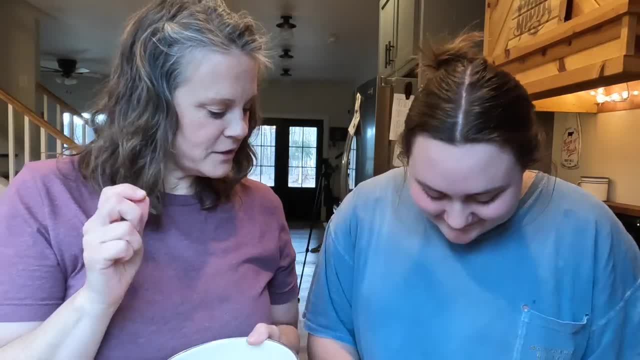 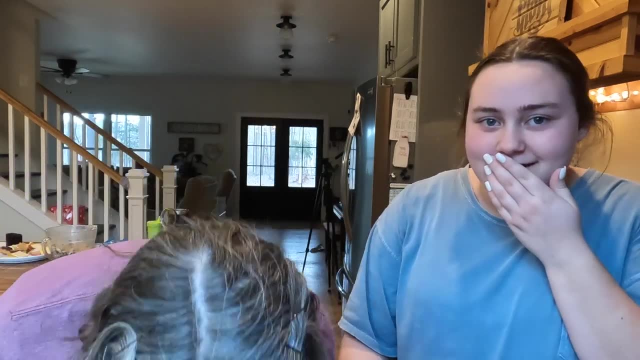 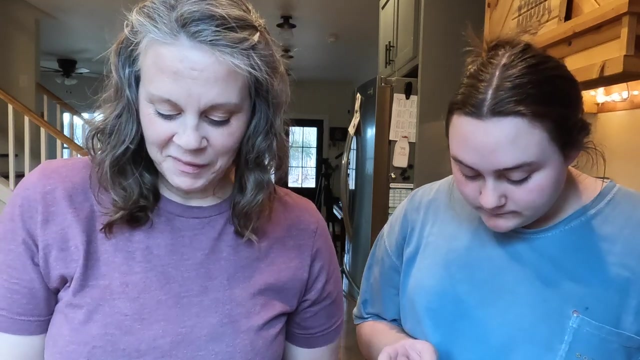 Kelsey and I are going to try our chickpeas. I just put salt on them. Mmm, It's not good. It's good. Maybe it's because I was starving. I would rather have something else, though. Well, I think they're good. 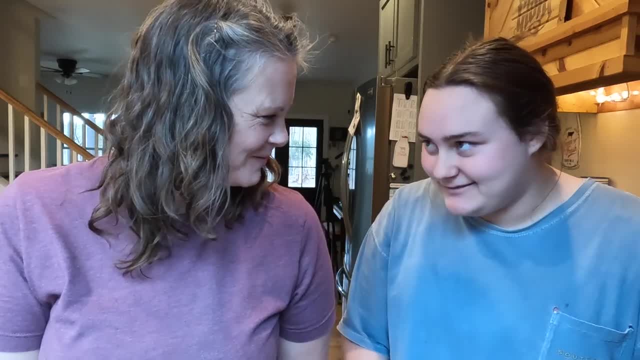 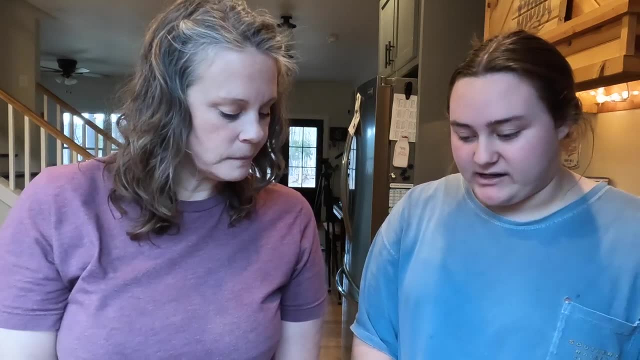 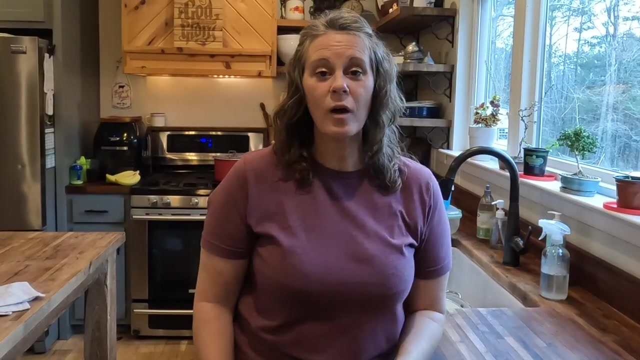 They're not terrible, Kenji's like boiled peanuts, but not as good. Mmm, I love boiled peanuts. Oh well, Kelsey's not a fan, but I am. A while back I was at Sam's Club and I saw that they had something called dill pickle dip. 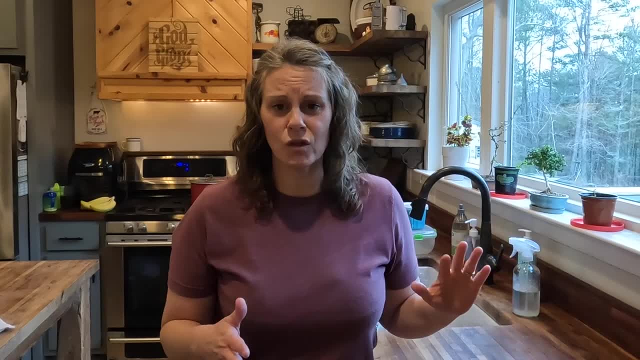 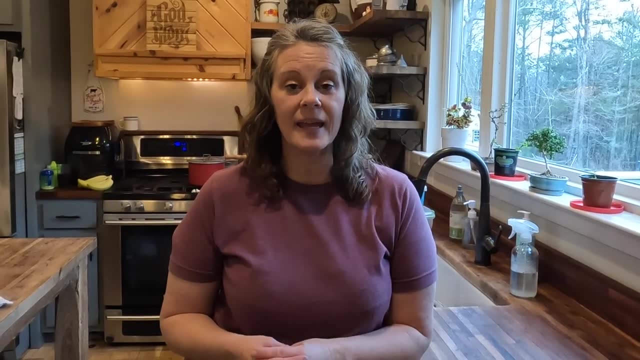 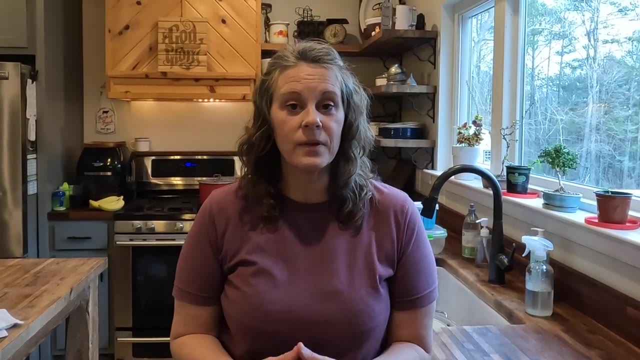 Mmm, That sounded so gross to me, Hmm, that I just scoffed and walked, walked away. but a few days later my friend had it at a party she was hosting, and so I gave it a try. no joke, it is one of the best dips I've ever had. so I'm going to share that recipe with you, and I promise. 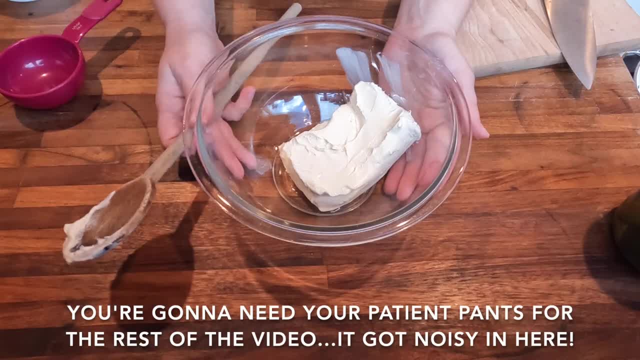 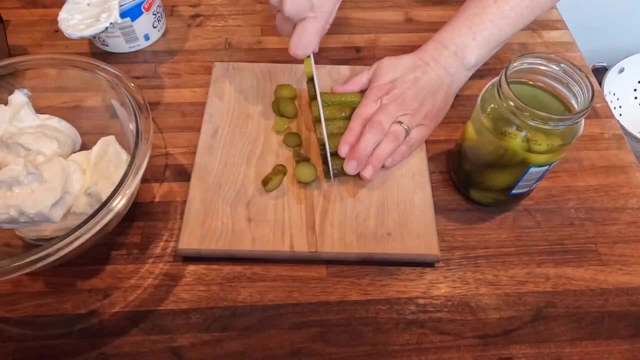 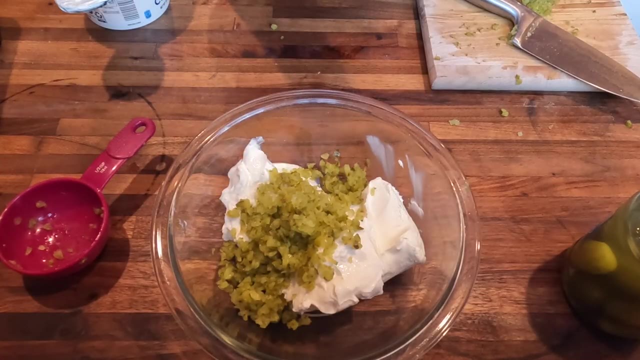 your family is going to love it. okay, for the dill pickle dip, we're going to use one block of cream cheese, one cup of sour cream, one and a half cups of chopped dill pickles. you might want to use a food processor for this. this takes a. 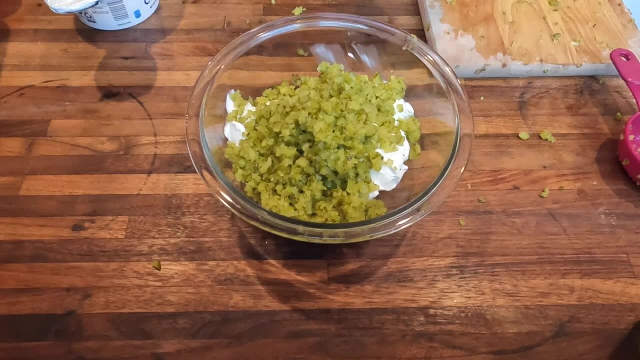 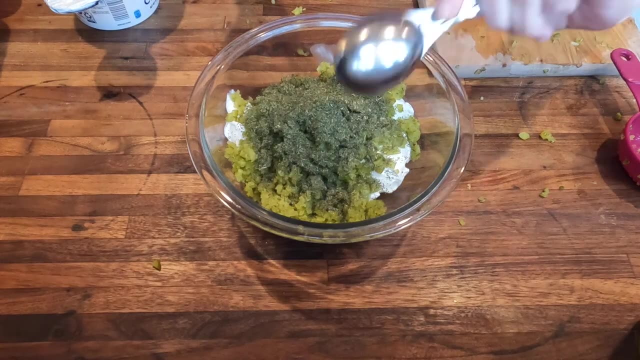 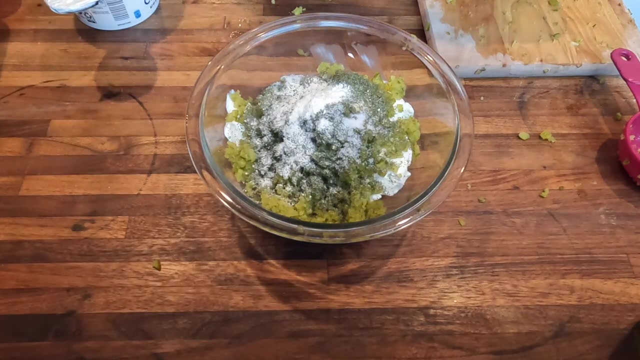 long time. to that we're going to start adding some spices, so we're going to add half a teaspoon of garlic powder, one and a half tablespoons of dill, a half teaspoon of salt, a teaspoon of dry milk powder and four teaspoons of pickle juice. I'm gonna give that a. 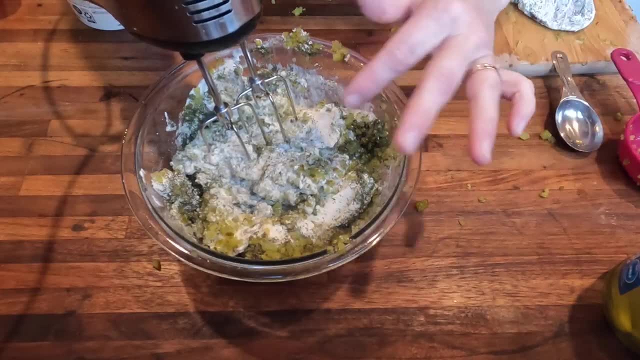 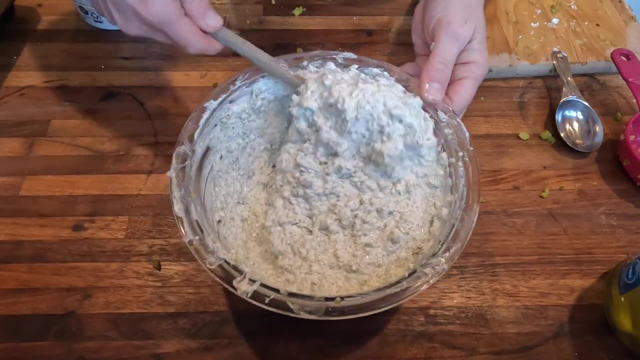 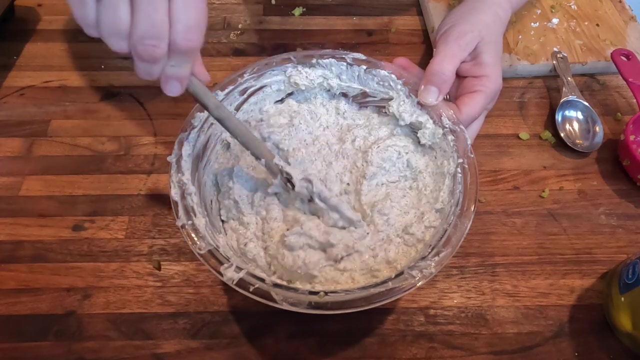 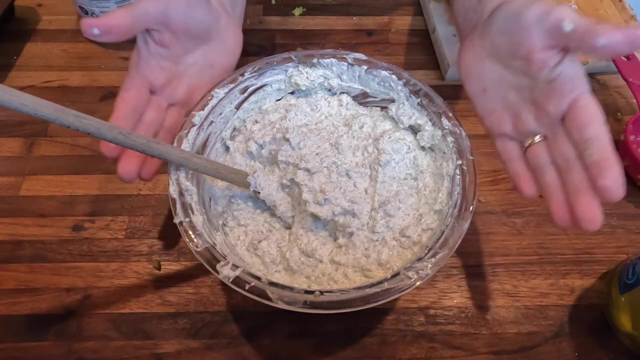 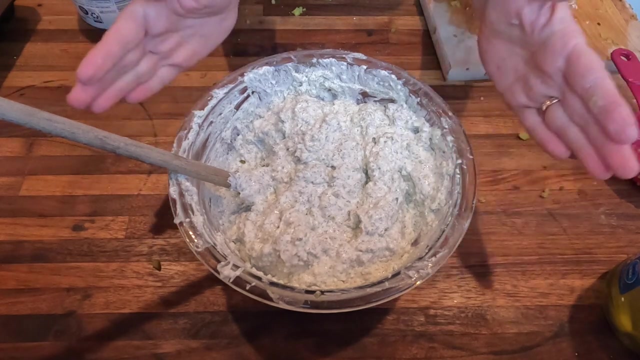 stir and then I'm gonna blend it with this mixer and there you go. this dip is going to be a serious hit. it's perfect for putting in your lunch with some candy carrots or some pita chips, or an after-school snack with some tortilla chips or even potato chips. I promise everybody is gonna like this dip well, I.